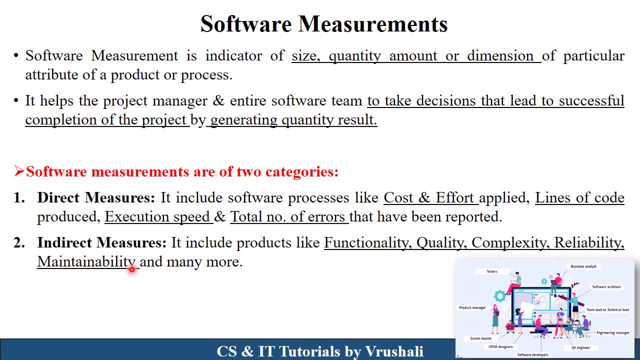 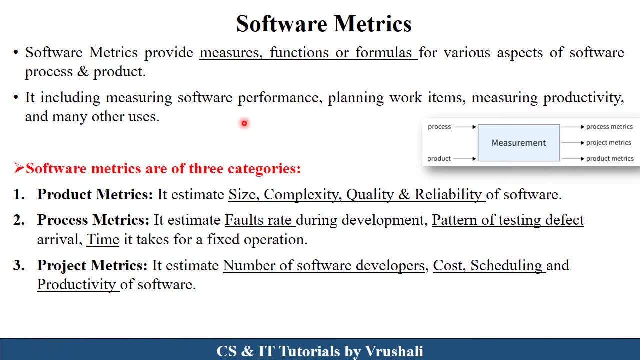 quality, complexity, reliability and maintainability of particular project. This kind of specification, So this is called as software measurements. The next topic is software measurement. So basically software metrics provide measures, functions or formulas to the particular software measurements. For example, in software measurement we calculate total number of errors occur in particular. 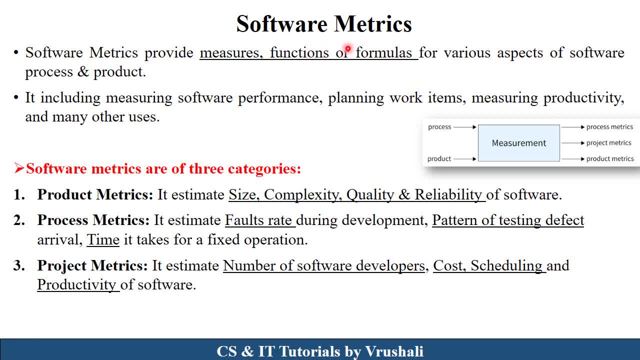 project. but in software metrics we provide a formula like total number of errors occur in per hour in particular project. After that they calculate total number of errors occur per day in particular project. so this is called as software matrix. software matrix measuring the software performance, complete planning of work items, then measuring productivity of particular. 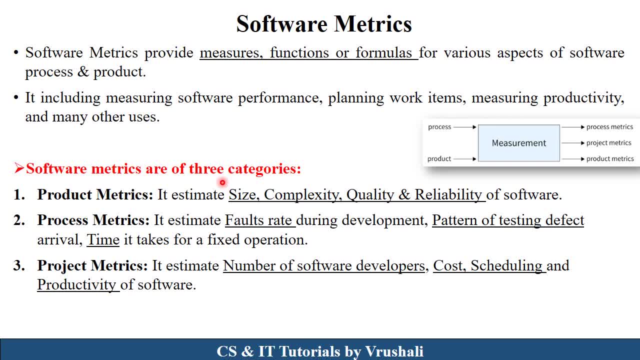 project software matrix divided into the three categories. like product matrix, which estimate size, complexity, quality and reliability of particular software, they provide functions and formulas for that purpose. the second one is a process matrix. here they estimate total fault rate, means how many bugs, how many errors and how many defaults are occurred in particular project. 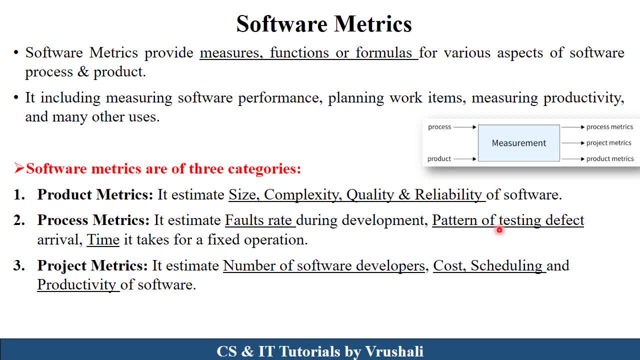 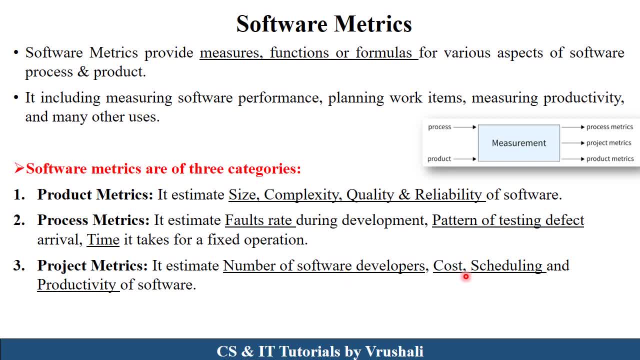 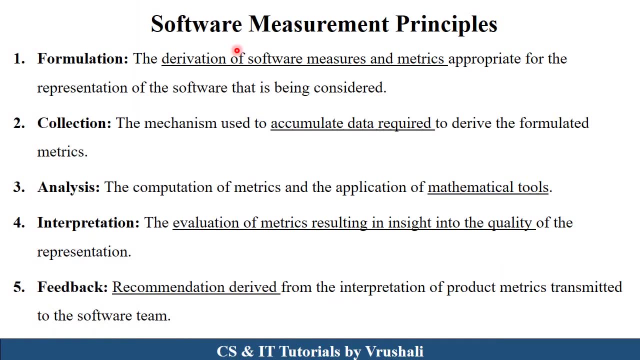 required for completing a particular project, then total number of cost, complete schedule and complete productivity of software. so this is called as software matrix. they provide measures, functions and formulas to the software measurements for calculating purpose. now the next important topic is software measurement principles. the first principle is formulation means here the derivation. 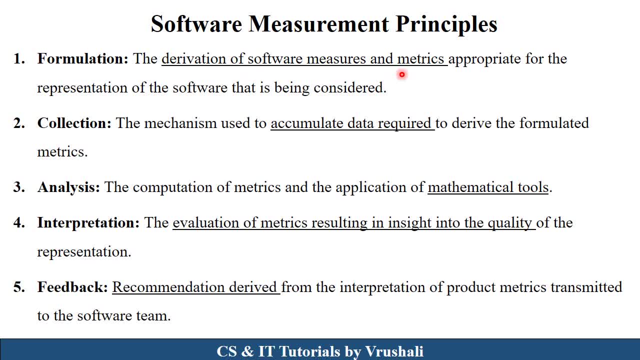 of software measures and matrix. for that purpose, different formulas are required and this formulas are applied on complete representation of the software. the second one is a collection. see there are different count or quantity have generated due to software measurements. so there is a lots of collections of data are required where different formulas have applied. next one: 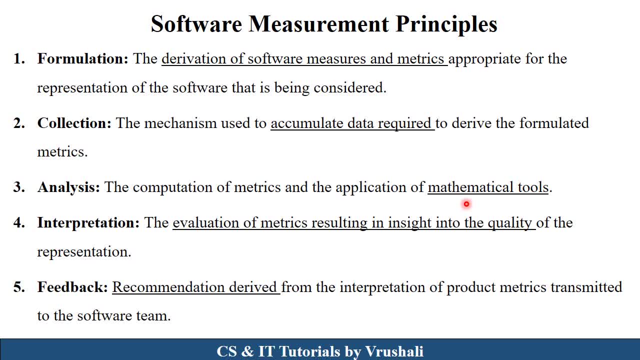 is the analysis there are in software measurement. there are different mathematical tools are used for analysis purpose. then interpretation: interpretation means after applying all the measurement formulas, they evaluate the quality of particular product. and last one is a feedback after interpretation, after generate evaluation, this particular data sent to the software team. 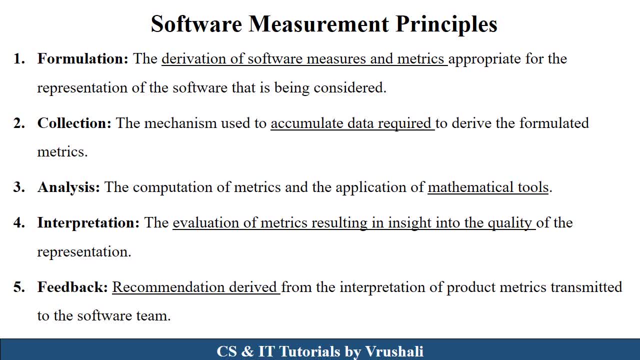 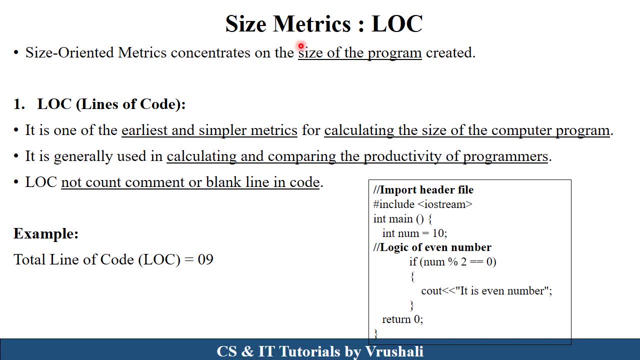 and software team feedback is necessary, that total number of cost time, then all the software measurements are good for particular project or not. so these are the principles of software measurements. now the next topic: size matrix. so there are two types of size matrix, that is, loc and fp. basically, this size oriented matrix focus on the complete size of the program. 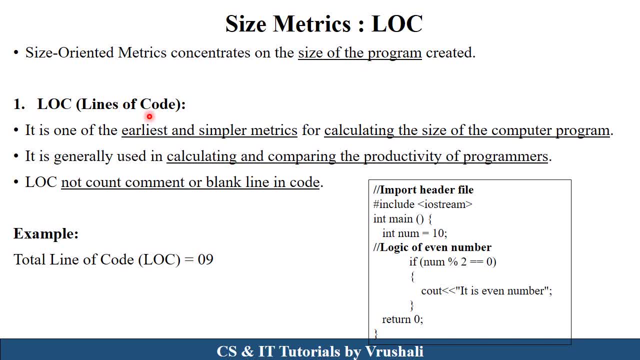 the first matrix is loc. loc stands for lines of code. it is one of the earliest and simplest matrix. they calculate complete size of your computer program. basically they calculate total number of lines for particular code. so it calculate and compare productivity of the programmers. see here, in this particular example, this is a simple, short program, that is, find out even numbers, ok, so 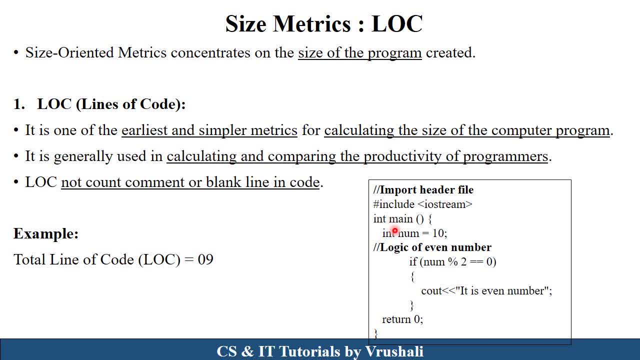 how many lines in the particular program? 1, 2, 3, 4, 5, 6, 7, 8, 9, 10 and 11. so there are total 11 number of lines here, but LOC don't count. comment or a blank line in particular code. 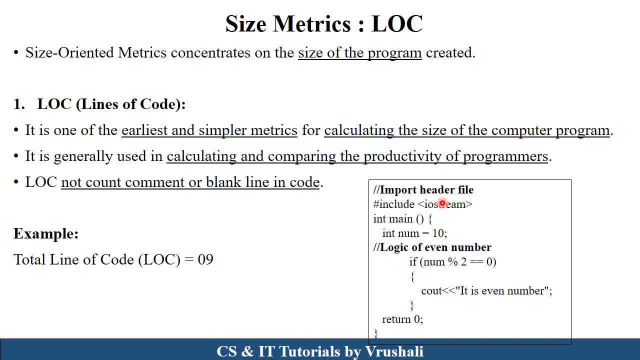 so there are 2 comments. line is here right, so 11-2, 9, so total line of code or total LOC in 9 in this particular program. similarly, this LOC calculate total number of lines used in particular project in complete project. so this is called as LOC. basically see here: 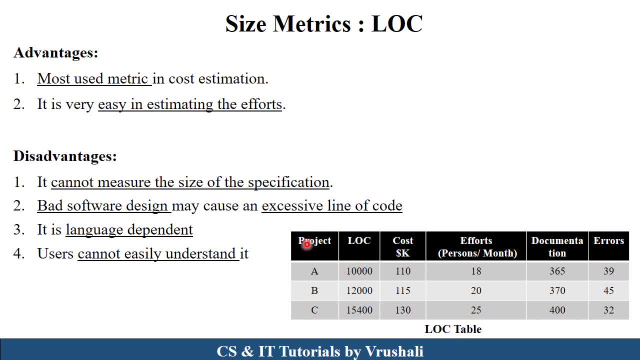 this is a LOC table. they calculate all these measurement. the first one is a project. suppose this is the first project. the project name is a in this a project. total number of lines of code is 10 000. then cost: dollar k means dollar k means after a dollar. one thousand line, before one thousand line. how much dollar is? 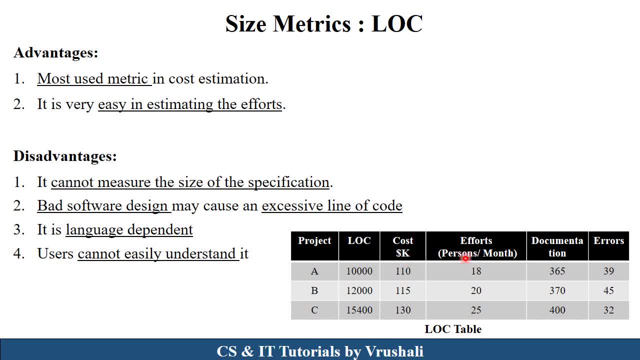 required. so one one ten dollar is required, then efforts means 18 percent per month is required for a particular project. then for this 10 000 lines of code, 365 pages are required, in particular documentation. and from this lines of code 39 errors have generated the. similarly with b and: 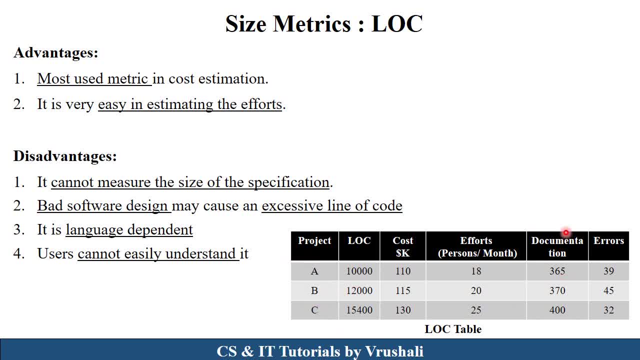 c project. so basically it measures all the loc details of particular project. the advantages of this size matrix is it most used matrix in cost estimation, it is easy for estimating all the efforts. but disadvantages are it cannot measure the size of this specification. they measure only line of code. then suppose there are some bad software designs, so there are. 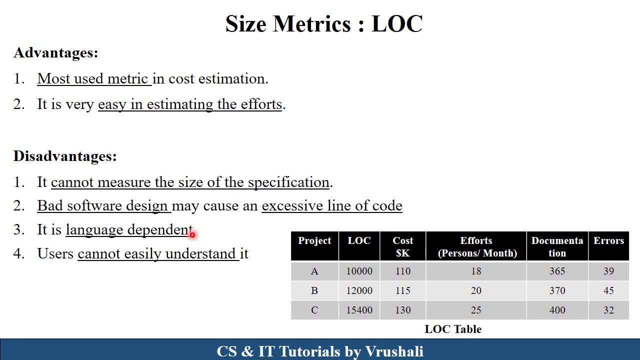 exceptions. there are some bad software designs, so there are exceptions. so there are some bad software designs. so there are some bad software designs. so there are some bad software designs. of course are present. it is a language dependent means. when you develop a particular project in c plus plus language, so for example, there are 10 number of lines are required. but when you develop 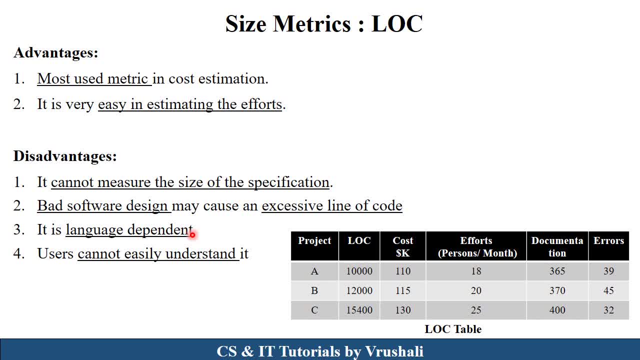 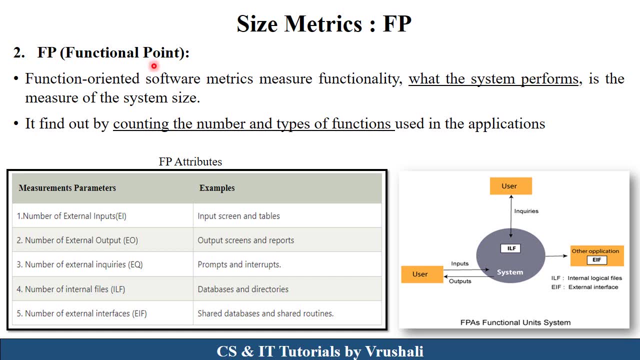 a same project in python programming. so there are only two or three numbers of lines are required, right? so it is a language dependent and user cannot easily understand it. all this cost estimation. now the second size matrix is fp, which is called as functional point. so functional point generally measure all the functionalities and what exactly system. 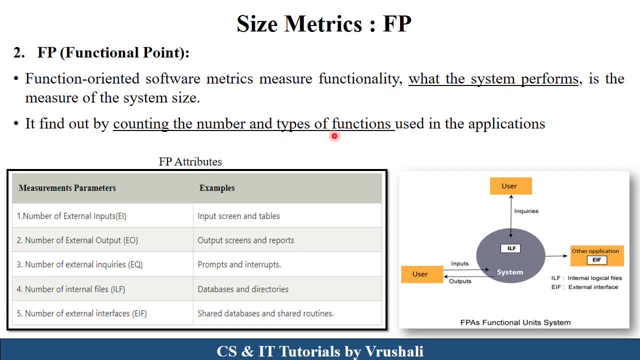 perform. basically it count number and types of functions used in particular project. see here in this diagram. this is a functional unit system. suppose this is your system, means your computer or your laptop. ilf means the number of internal files in particular system. now user. so user interact with particular system. user sends some input through keyboard. 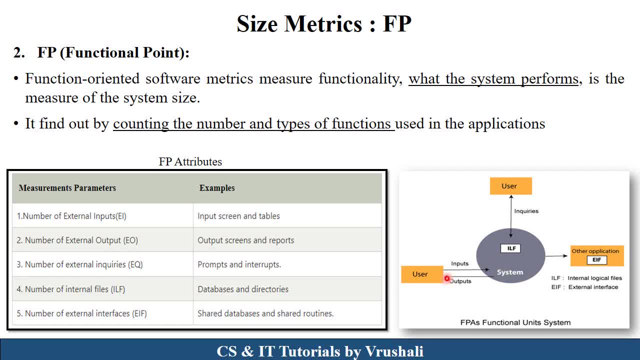 and mouse. then system give output through your the particular monitor screen. right now user inquiry sent to the particular system like there are some errors or interrupts are generated some inquiries or helping system is there. now there are other application. other application means eif means number of external interfaces. sometimes you can use external devices like database, external mouse. 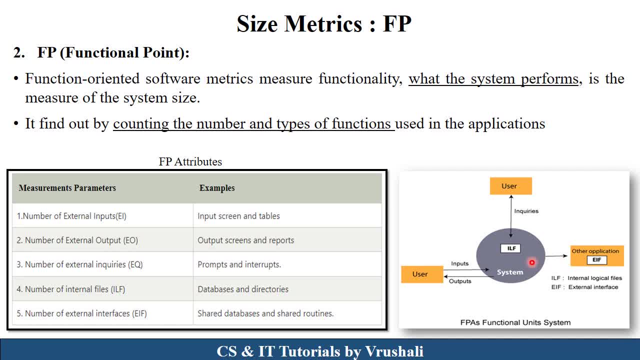 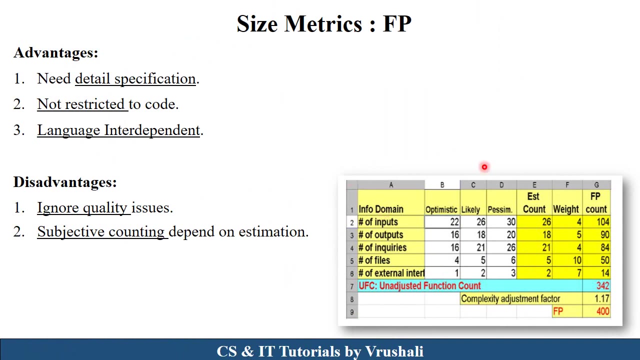 external, uh, hard disk is used for particular system, right? so basically, functional point: calculate all those things. they calculate number of external inputs, number of external outputs, then total number of inquiries, total number of input and outputs and total number of external interfaces. they calculate all those things. now this fp generate this kind of table by calculating all the specification of particular. 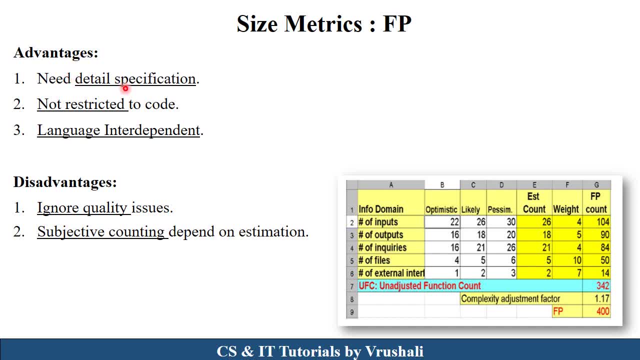 system. the advantages of fp is they need a detailed specification. they calculate what exactly input and output send towards a particular system. there is not restricted towards the code because they work on specification or operations. this is language interdependent. but the disadvantages are they ignore quality issues. they calculate overall steps. they ignore. 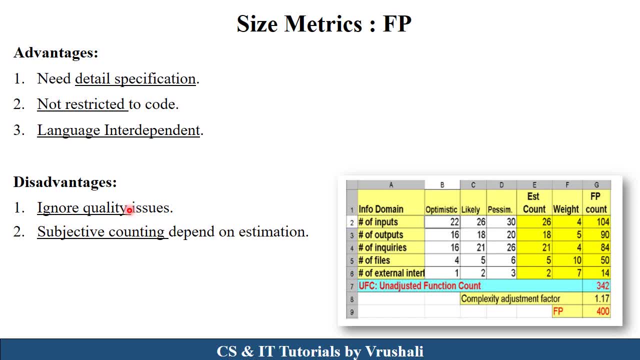 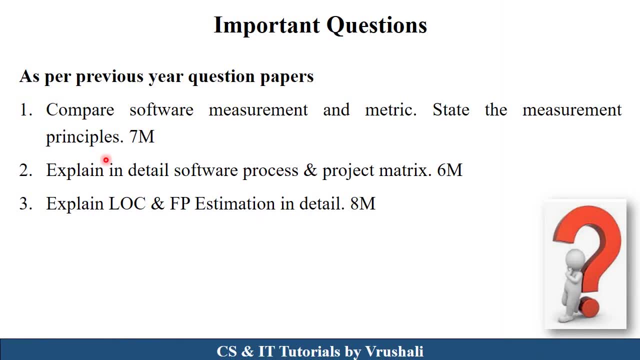 quality issues. they only focus on all the functionalities and there is a subjective counting, depend on estimation. so these are the disadvantages of fp. now, as per your previous year, these questions have asked like: compare software measurement and matrix state. the measurement principles for seven marks explain in detail software process and project matrix for six marks. 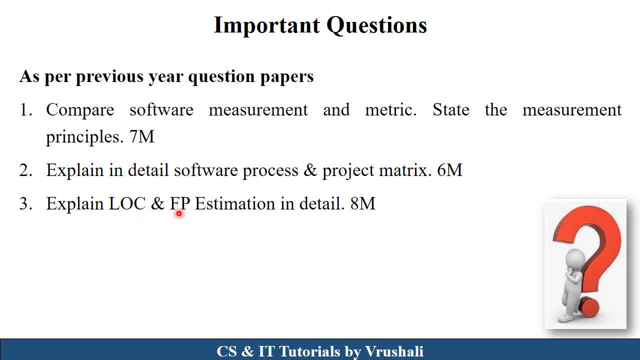 and explain alloc and fp estimation in detail for eight marks. so you have to prepare this topic. so thank you, keep learning.